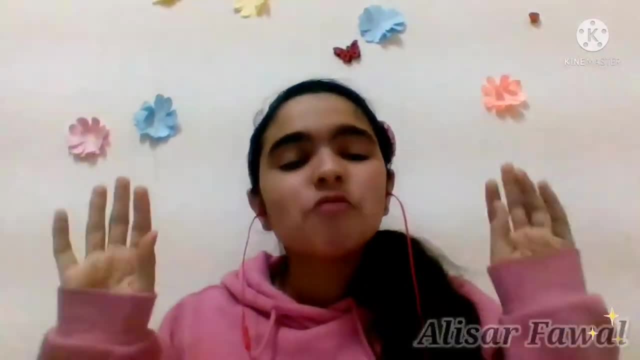 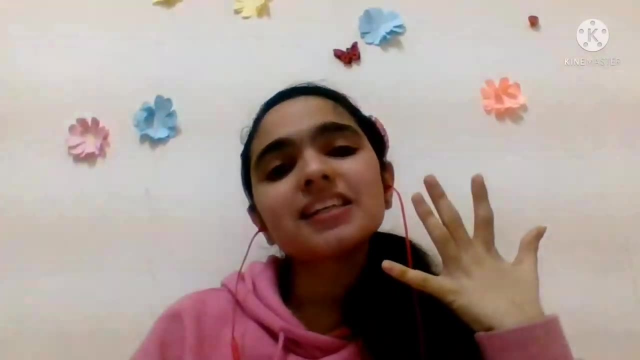 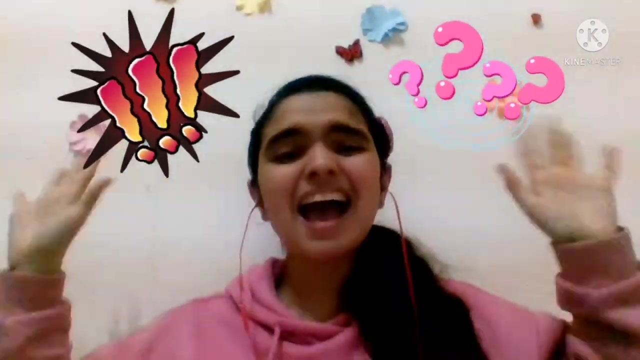 I'm Alisar from 11A and today we will talk about acids and bases. But wait wait wait wait don't read. Acids and bases might sound like a complicated topic and some of you will be like acids are corrosive. But today there's something different. We'll be having something interesting 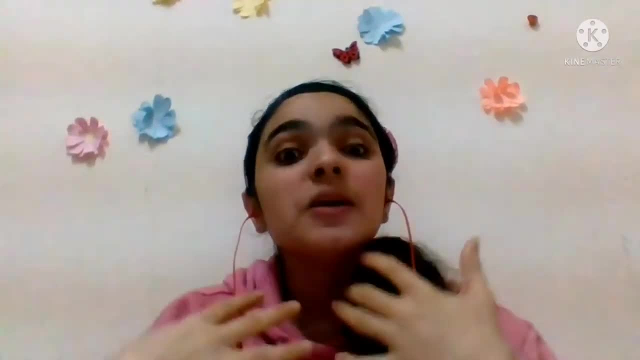 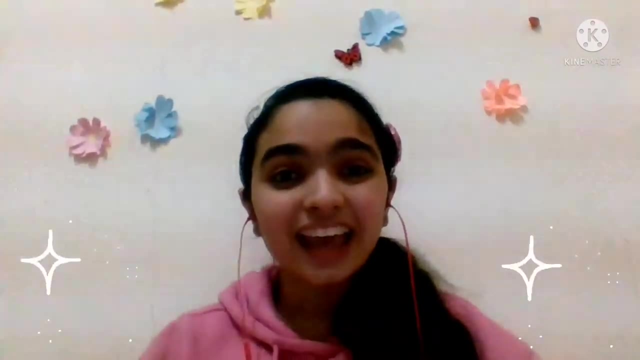 and unique. Do you know that us as humans we use acids and bases in our daily life? Yeah we use it like literally every day. How and when? Well keep on watching to know more. 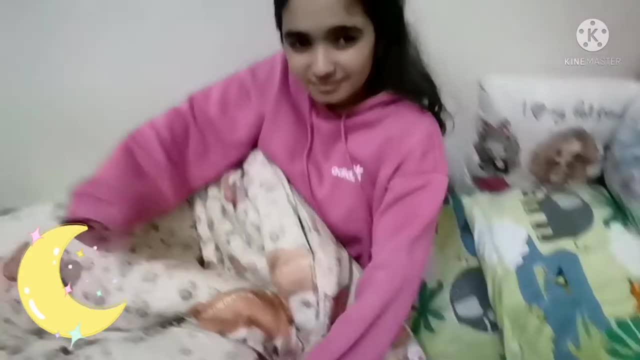 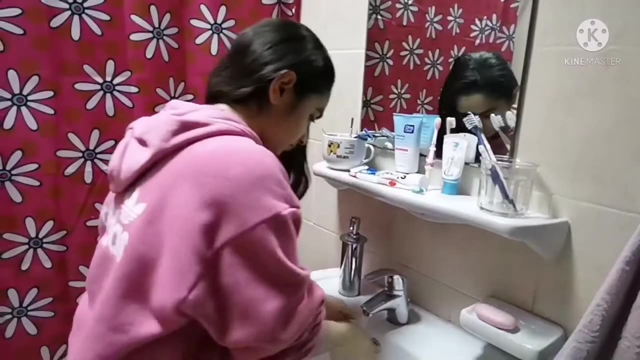 Let's start when you first wake up and open your eyes. Shiny morning! Now go wash your face and get ready. 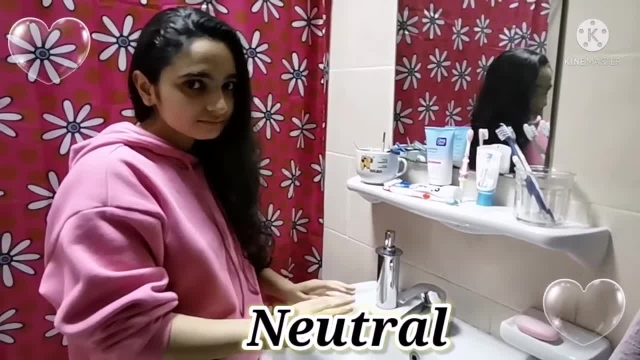 Don't worry don't worry water is not acidic nor basic it's neutral. Now that you washed your face I think you're ready to brush your teeth. 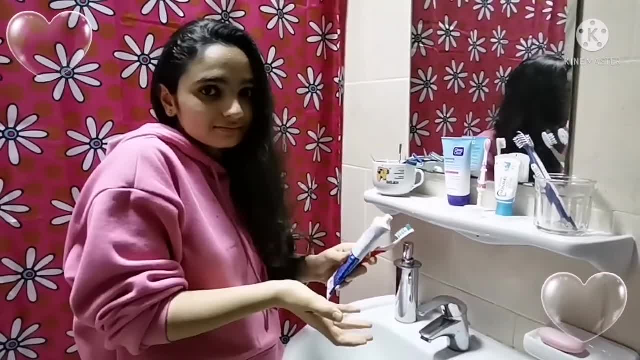 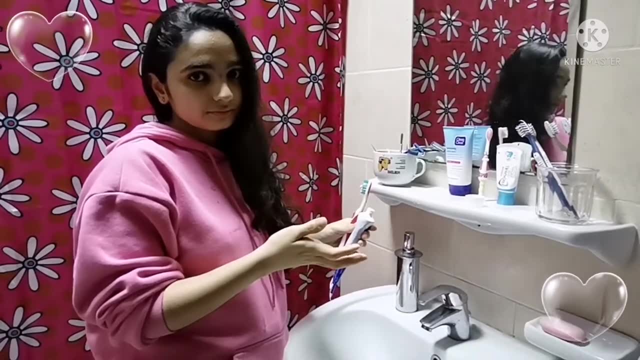 Oh look at this you're using a toothpaste and you know what? A toothpaste is a base that has a pH of 8 or 10. Okay now you can brush your teeth. 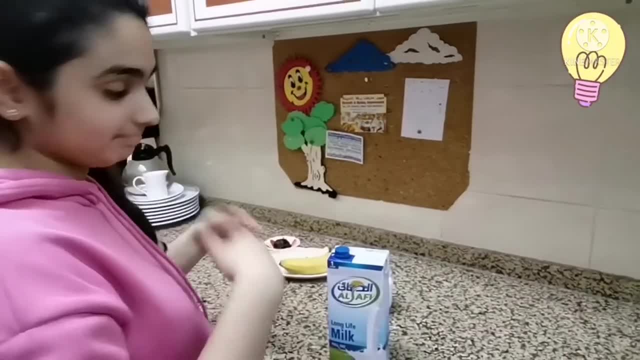 What are you thinking about now? Oh you're gonna have breakfast! First, what's on the list? 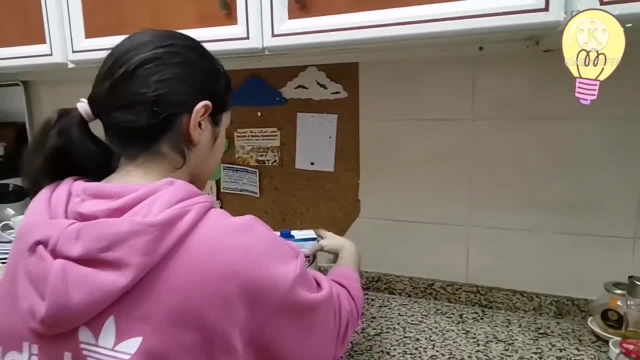 Ooh, you'll be having some milk? You know what? Milk is acidic too. 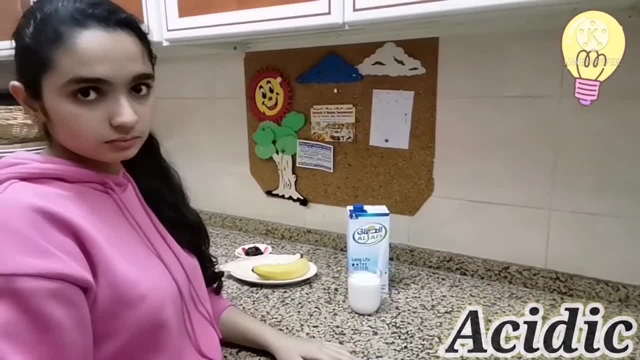 Yeah, it has a pH of 6.7 to 6.9. So don't really worry, it's not that acidic. 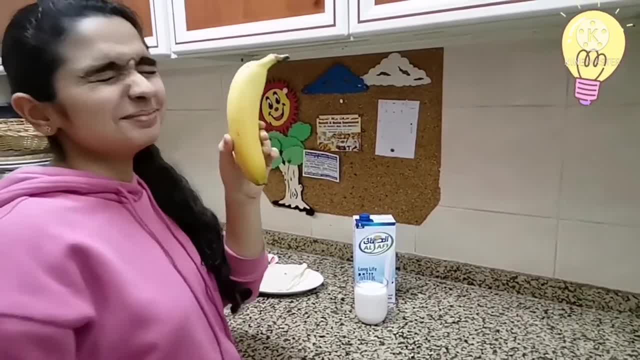 What's next? A banana? Such a healthy decision. 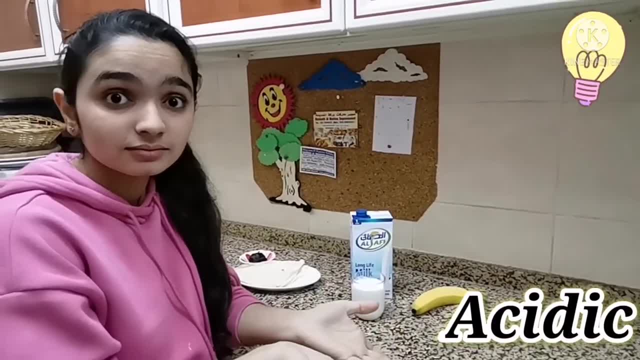 Although it's slightly acidic with a pH of 5, it's a healthy decision and full of proteins as well. What's next on your breakfast list? Hmm, you'll be having some bread? 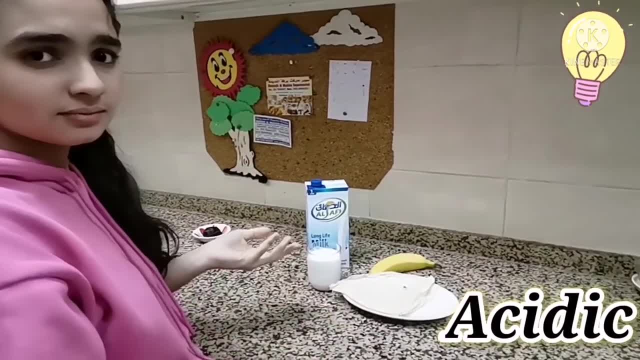 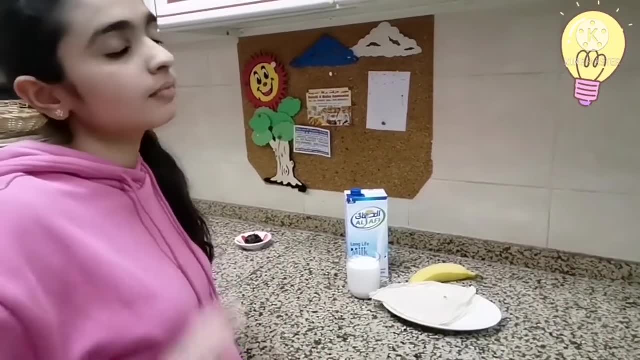 Bread is slightly acidic with a pH that is usually ranging between 5 to 6.5. So it's a bit, don't worry, it's not that much acidic and it's still really healthy. What else? 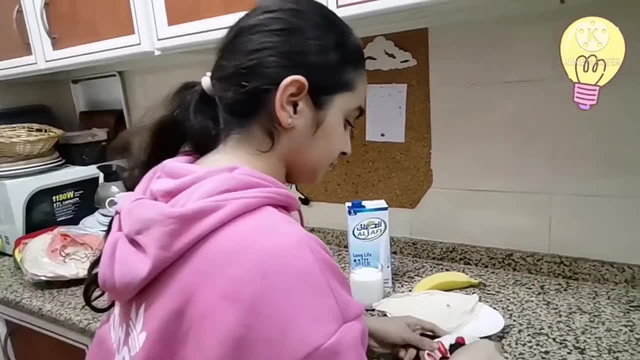 Of course, you'll be having dates. You live in the UAE. That's logical. 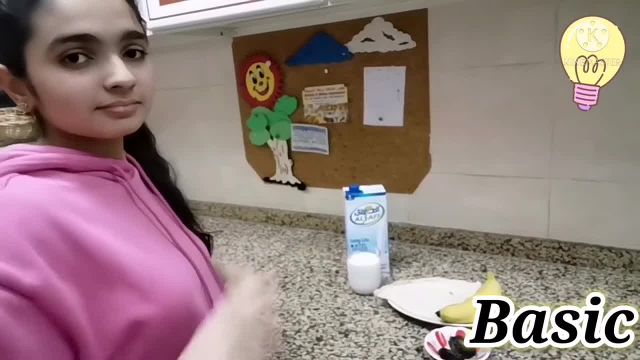 Dates are one of the highly alkaline or basic fruits with a pH level of 6.5 to 8.5. And it's super duper healthy. Okay, have a nice breakfast. 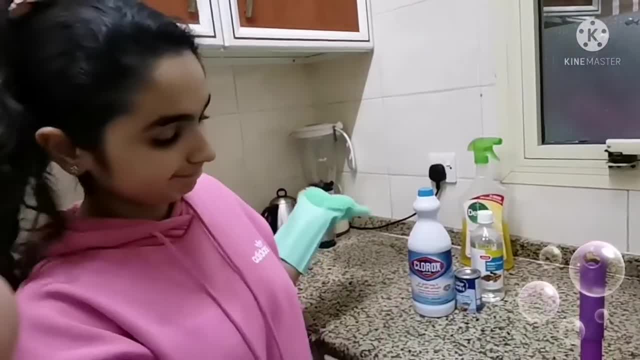 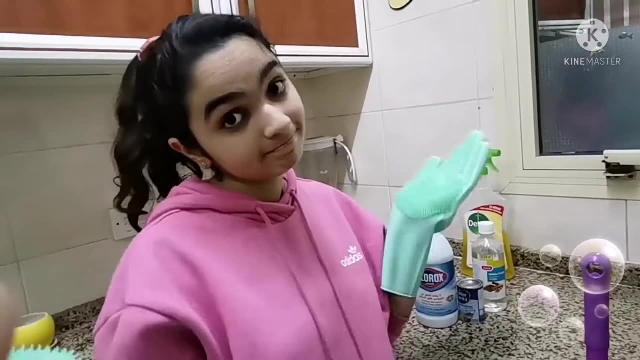 So, what are you planning today? Oh, you'll be doing a full clean up for your house today? Okay then, that's great. Hmm, you'll be using Clorox? Hmm, well, that's actually a basic material. What, for the carbonate soda beside it? It's acidic with a pH of 3 to 4. What? Vinegar? Why would you use vinegar? Oh, you're curious. 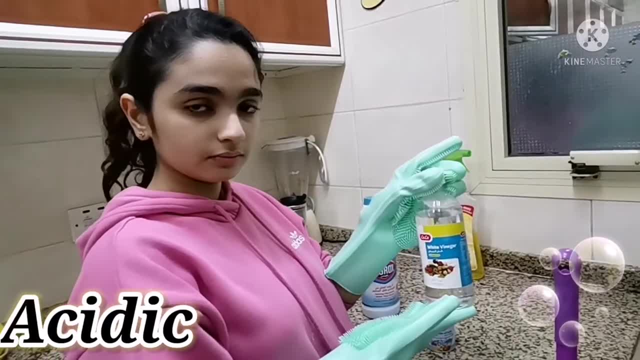 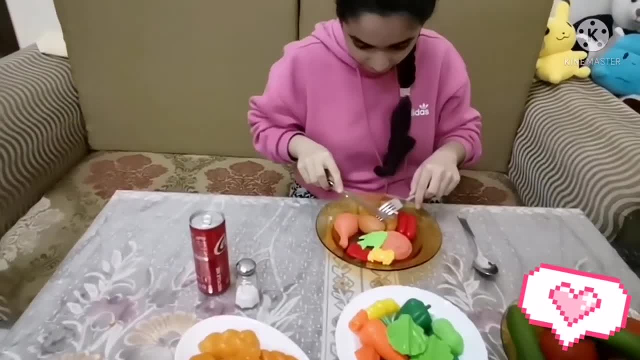 Hey, hey, hey, what are you eating? I want to see, I want to see. Ooh, you're having some meat? 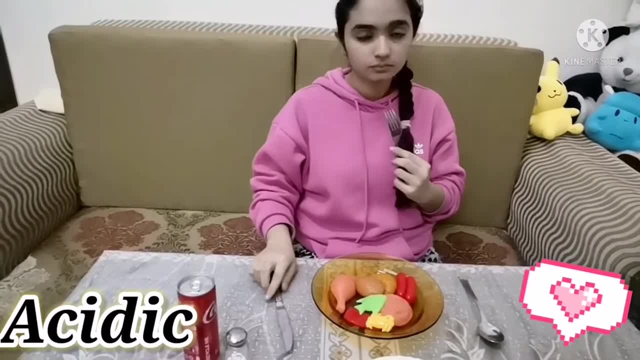 Well, do you know that meat is slightly acidic? What else? Yummy, you're having some salad. 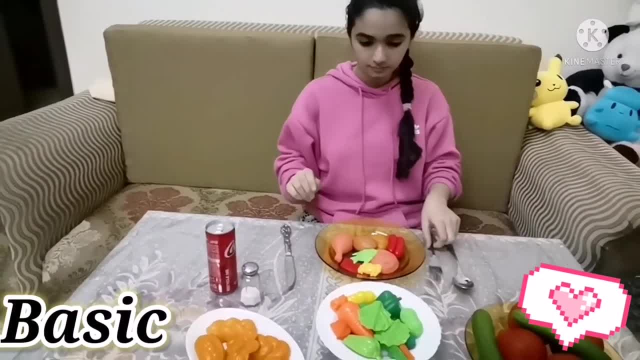 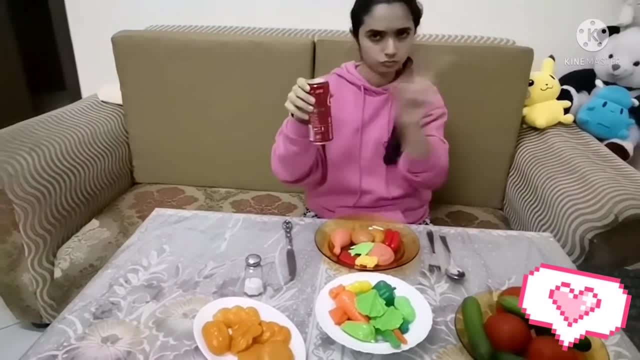 Vegetables, generally, are known to be basic and healthy, of course. And we all know that a salad is a healthy food. And we all know that a salad is much better than having a soft drink, since a soft drink is acidic and it's full of sugar. Great job, you're such a healthy girl. 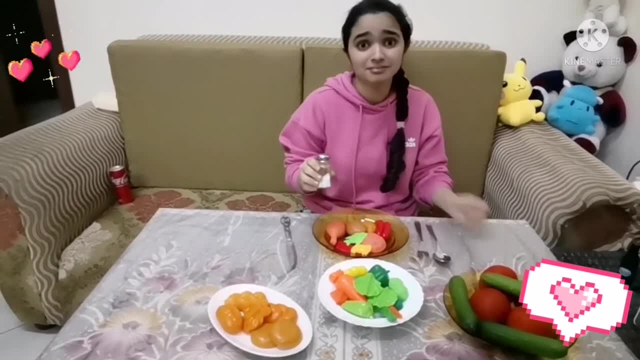 Oh, that's some salt? Do you know that? Oh, no, no, don't worry. It's neutral. 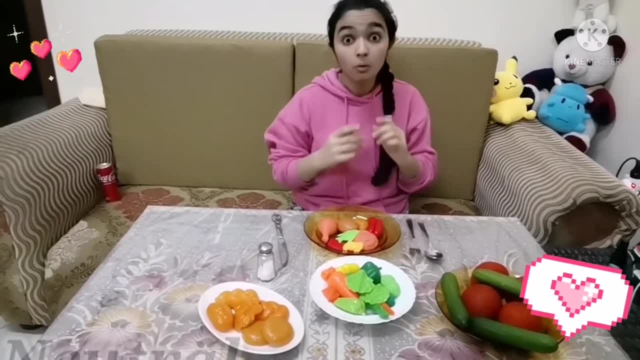 But because it's a mixture of acids and bases, just like water. Where are you going? 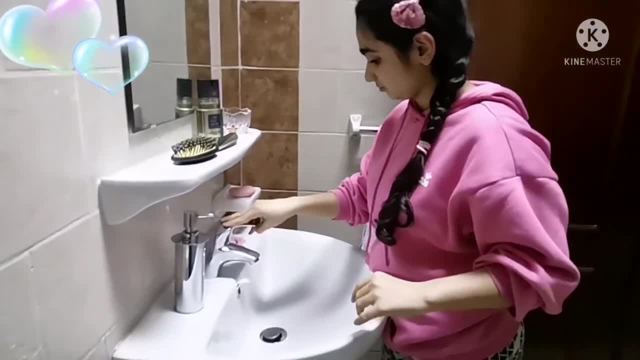 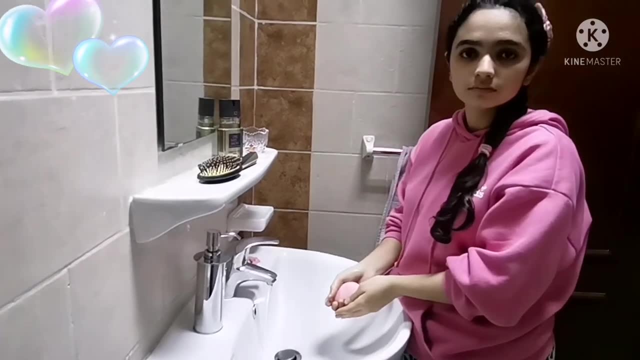 All right, you'll be washing your hands. Look at this. You will be using basic soap, which has a pH of 10. Fine, fine, I'll let you live in peace and wash your hands. See?